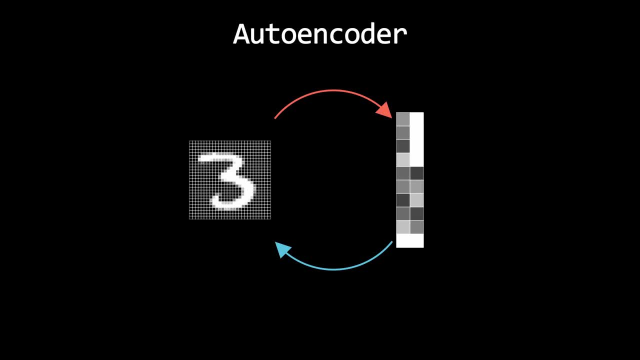 or forth and back operation. We encode in one direction and then we want to go in the opposite direction and decode it again to get the original image. So for each transformation we apply in the encoder, we want to apply the inverse of this operation in the decoder. 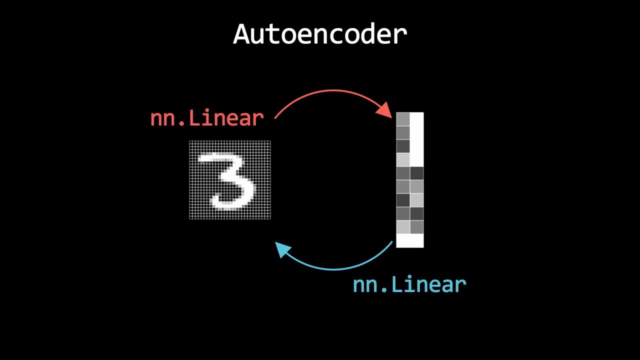 For example, if we apply a linear layer that reduces the size, the reverse operation is also a linear layer that increases the size again. Now for CNNs. this is a little bit trickier. Here we apply convolutional layers, so the inverse is actually called a transpose convolution. PyTorch has this layer already. 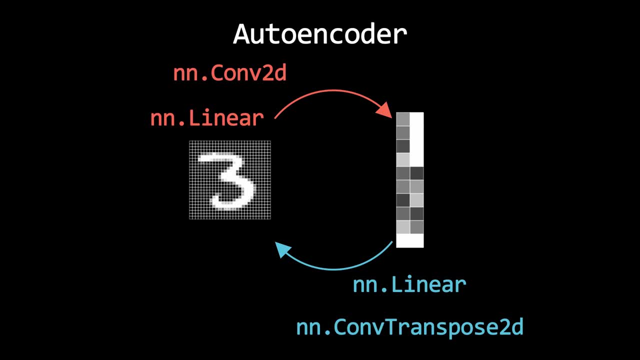 included for us, so we can simply use the nnconf transpose 2d layer. The only tricky thing with this is to determine the correct input and output shapes, but I will show you how to do this later. Alright, so that's everything we need to understand. autoencoders. Now we can jump to the 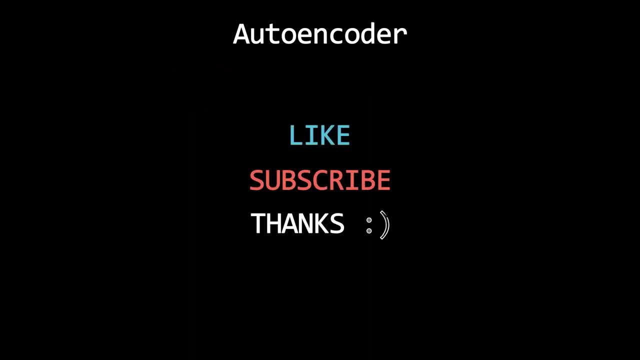 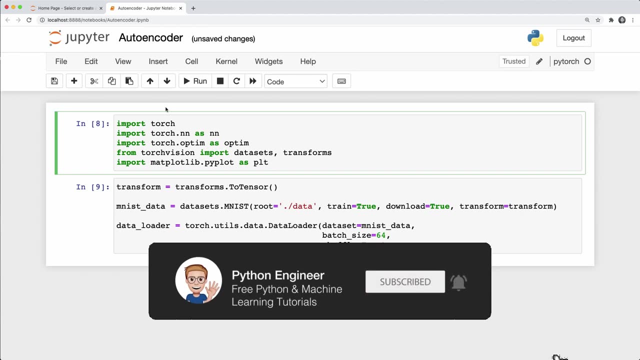 code and if you enjoy this content, then I would be very happy if you hit the like button and subscribe to the channel. Alright, so here we are in a Jupyter notebook and we already have all the imports that we need. So we have torch, we have torch nn, torch optim, we have datasets and 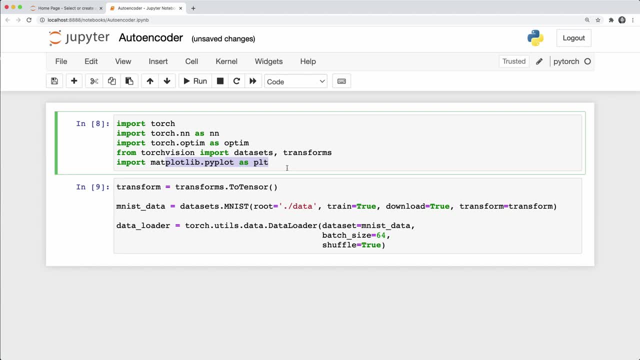 transforms from the torch vision module and we have matplotlib to plot the data later. And then the first thing we want to do is load the MNIST data, And for this we use a data loader. And if you don't know how a data loader works, 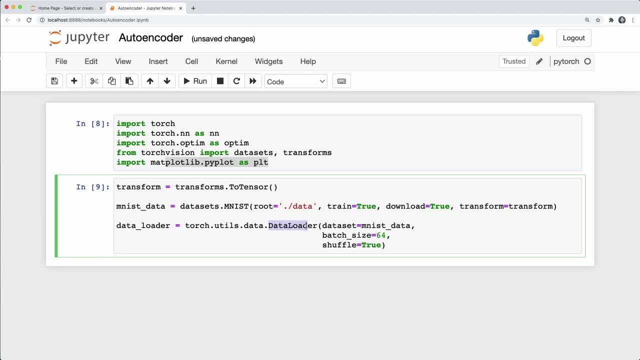 then I will link a tutorial where I explain this here. So we define a data loader and we can give it a batch size here And we also define the data set. So this is included in PyTorch And we get this by saying datasets dot MNIST And this will download the data and store it here in the data. 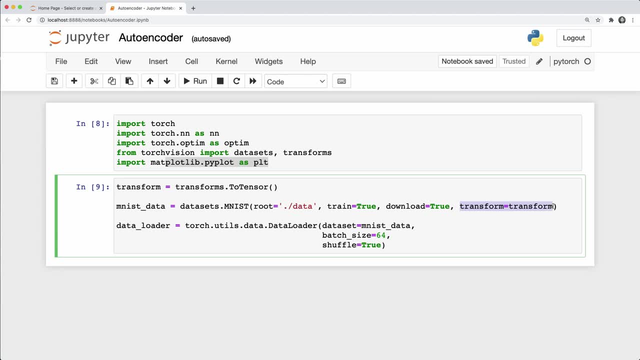 folder And we also can apply a transform here, and in this case we simply apply a to-tenso transform. so this will transform the images to a pine torch tensor, And I pulled this out here because this is actually important for our model later. 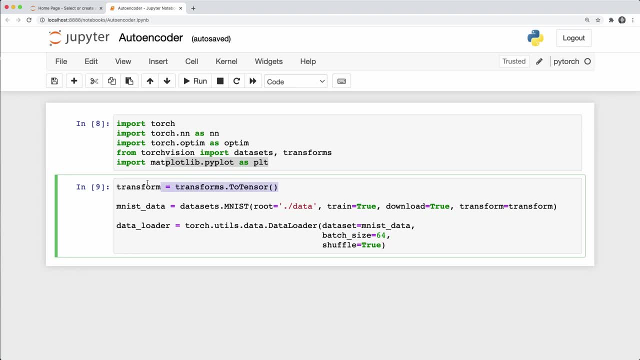 So later I also wants to show you what we have to consider when we use a different transform here. So we will get to this later, But for now what we want to keep in mind. So we will call to this later, But for now what we want to keep in mind. 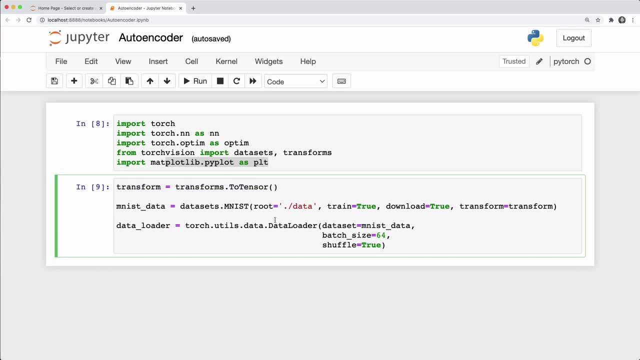 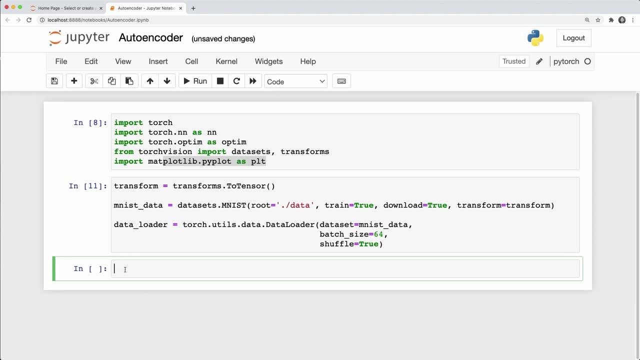 is how our data looks like. So what values do our MNIST images have? So let's actually run this and let's inspect the first images or the first batch. So we get the first batch by creating a iterator object like: so we say data iter and then we call iter with our data loader And then we pull. 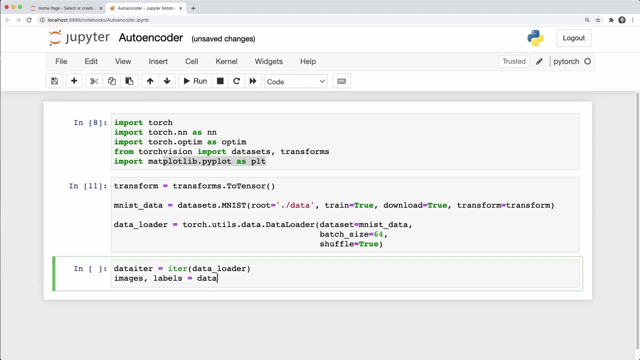 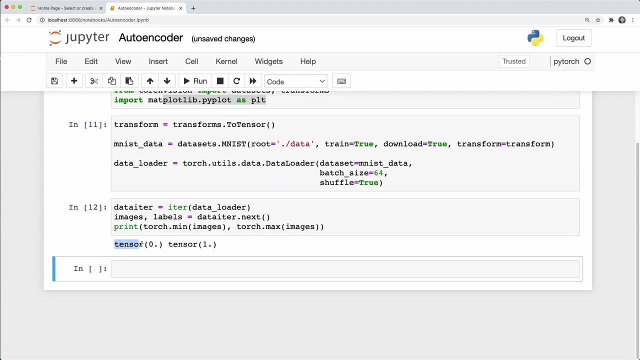 out the first images and labels by calling data iter dot next, And then we want to print the minimum and the maximum value and we get this with torch dot min of our images and also torch dot max of our images. So let's run this And then we see the values range from zero to one. So this will be. 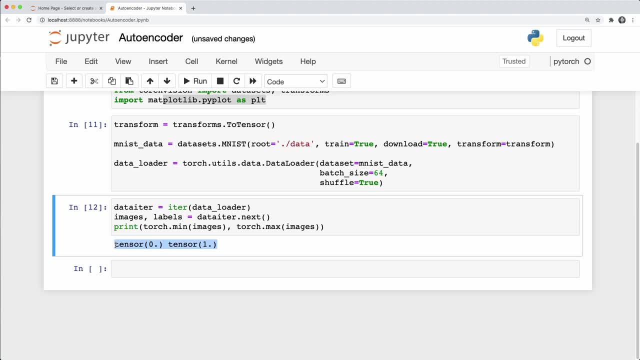 important for our model later, And this might change if we also change the transforms here. So we will learn how to do this later. So, with this in mind, that the values are between zero and one, we can create our auto encoder class. 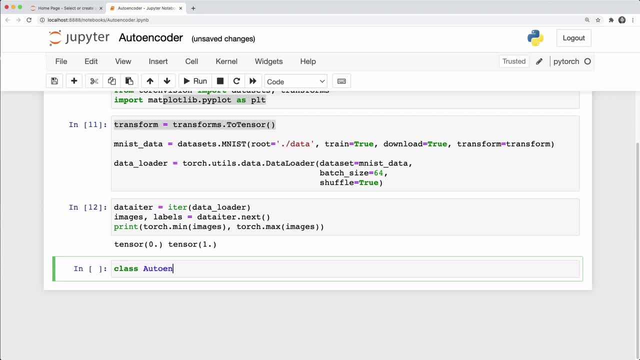 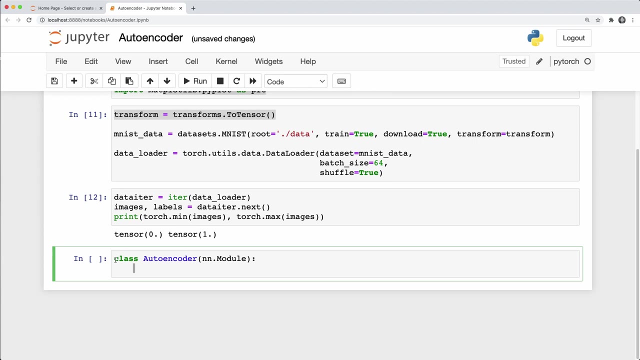 So let's create a class And let's call this auto encoder, And this is our model. So we have to inherit from nn dot module And if you don't know how to do this, then I will link another tutorial here where I explain how you create your pytorch classes. So the first thing we want to implement: 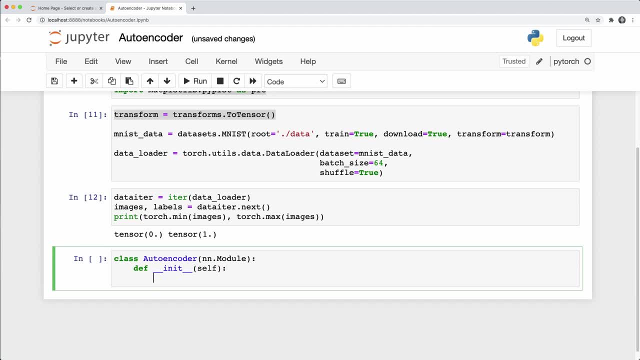 is the init function, And this only gets self. And then we also want to implement the forward pass, And this gets self and x. So for now we only say pass. And in the first example I want to show you a simple feed forward neural net with linear layers and a few hidden layers. 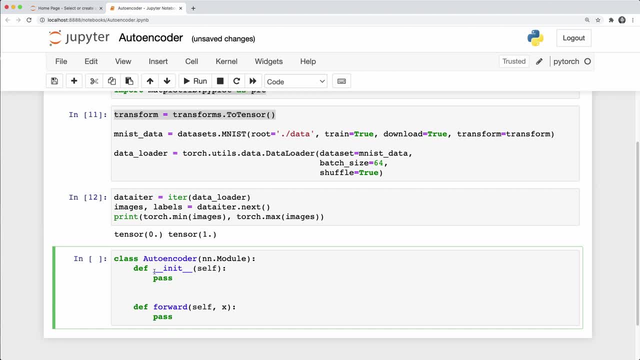 And here what we want to do is we want to repeatedly reduce the size. So in the beginning our images have the size n, and then by 784.. So this is 28 by 28.. Because this is how many pixels the images have in this. 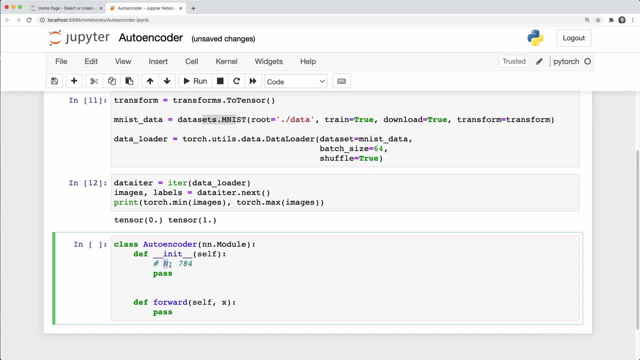 data Is that, And n is our batch size. So now we want to reduce this with a few linear layers, And a good way to structure your code in an auto encoder is to use a sequential model. So first we create a n coder and this is a n n dot sequential model. And now here we want to. 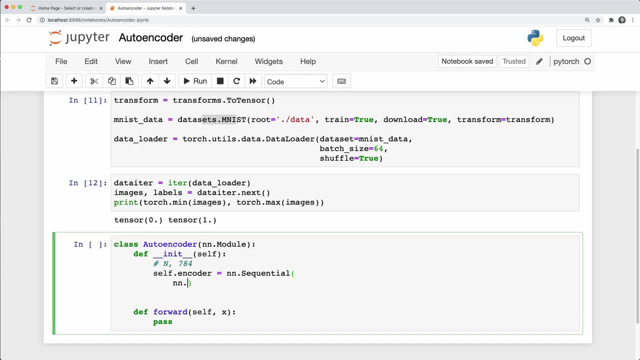 repeatedly apply linear layers. So let's create a first linear model And we will create that, and we will define that as partial model. And an auto encoder was intended for the order of order, So let us call thisays你的 entry data set and phrase. coder is equal to sign in dot en female code n en 60 to인words. 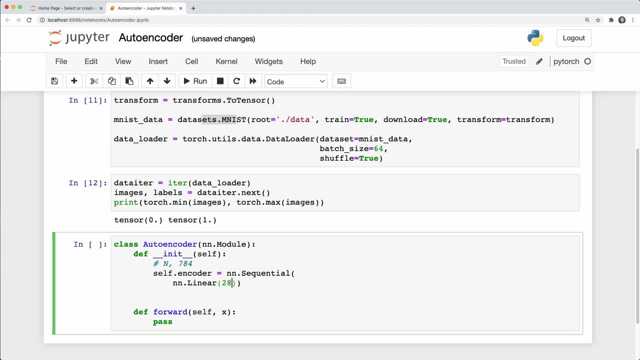 Curve. What's your code file like? Well, this is the URL of your code file, but let's� Al裡面 input a few comments here too. first, linear layers, and the input size is 28 by 28.. So this is 784.. And the output size. 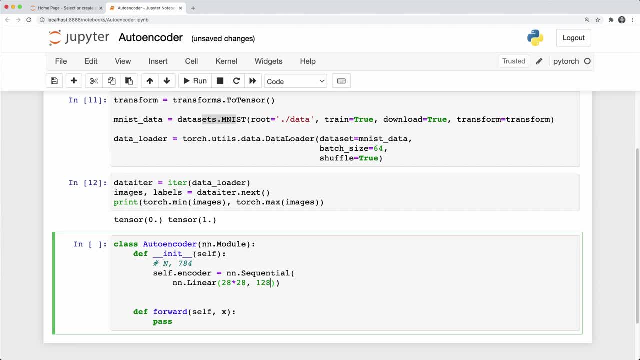 here we can play around with different sizes. So as first output size, I want to use 128.. So what this is doing is this: will reduce the size from n by 784, will reduce it to n by 128.. After this we also want to apply a activation function. So here we use nn dot. 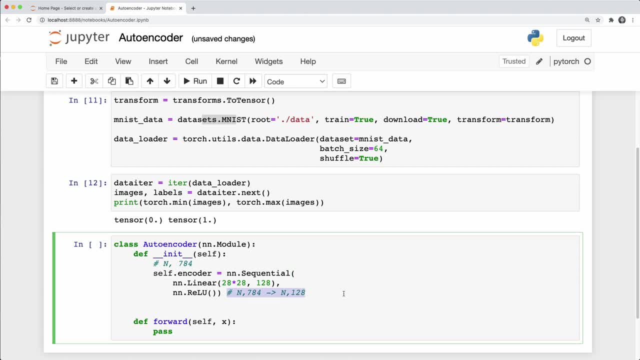 relu, the most popular one, And let's move the comments up here again. And now we want to do this multiple times. So so now we want to create another linear layer, And this time our input is 128.. And as output: 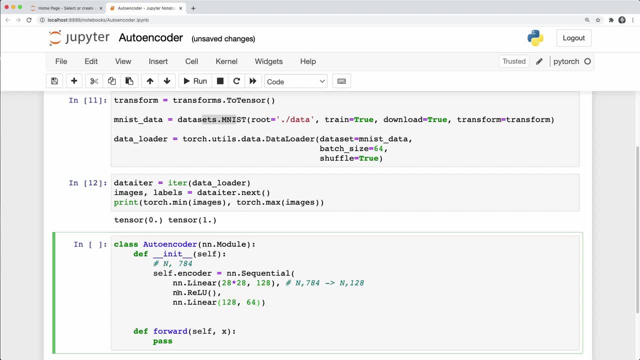 we can choose a different, smaller size. So here I use 64. And then again we want to apply the relu activation, And then let's do this a couple more times. So let's actually copy and paste this, So we create another linear layer. 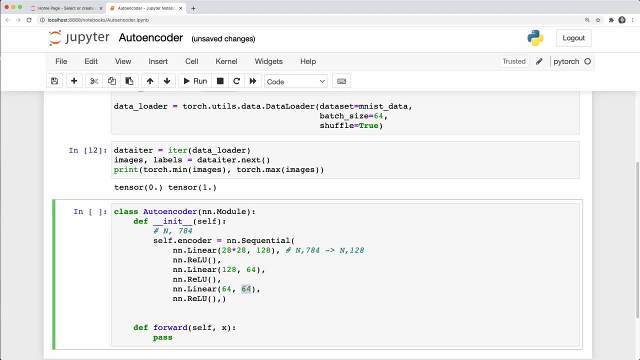 And here we use 64.. And as output, let's use 12.. Then again we have the relu, And now we create one last linear layer, So nn dot linear, And here we use 12.. And as output size, let's use three. 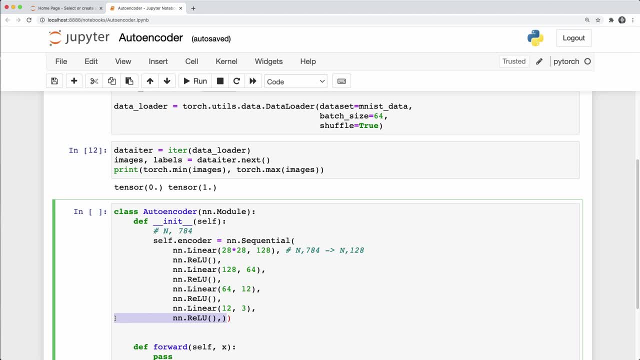 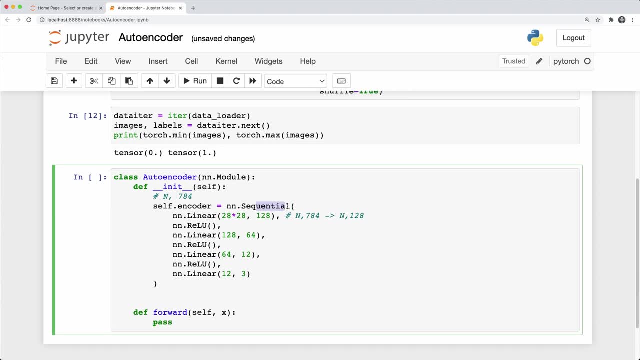 And then, as the last layer here, we don't need an activation function, So let's remove this again. So now this is our sequential model for the encoder, And the final output size here is n by three. So this will drastically reduce the size of our input images from this size. 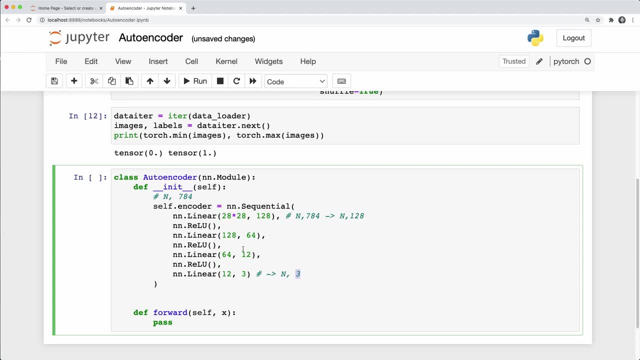 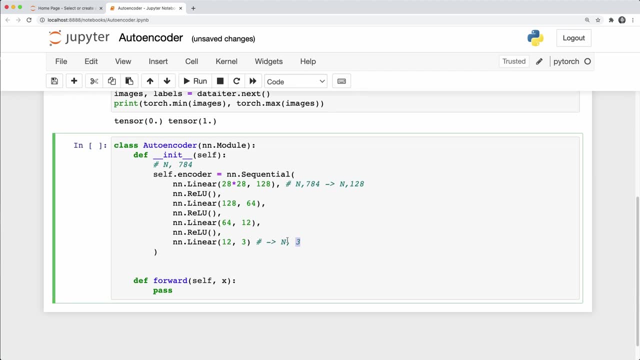 to only this size, And then later we are able to almost perfectly reconstruct this again. So this is really great. So, yeah, this is our encoder, And now we want to do the same thing in the opposite direction. So let's copy this actually and say: this is our self. 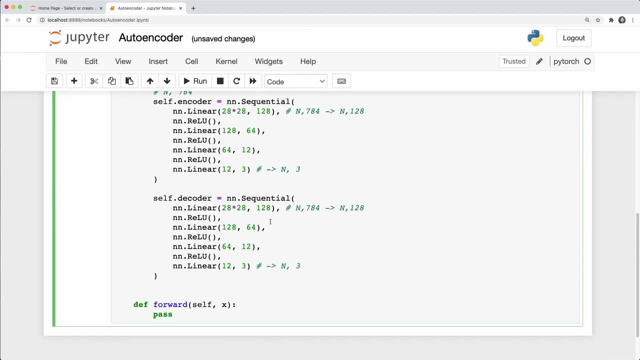 dot decoder. So here we want to go in the opposite direction. So here we want to go from n by three all the way again until n by 784.. So let's remove the comment here. And so now we basically we want to look at all the limits. 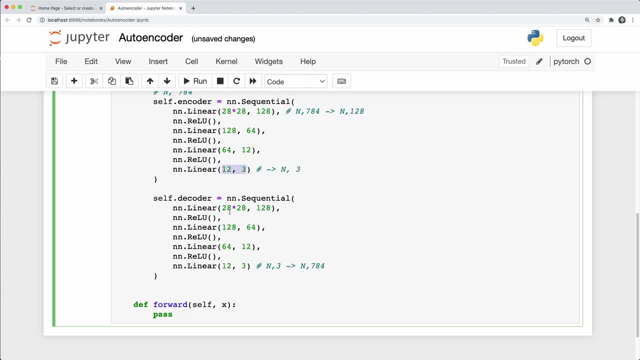 the linear layers and switch the sizes. So here the input size is three and the output size is 12.. Then here we have 12 and 64.. Here we have 64, and then as output size 128.. And here we have 128 and as output size 28 times 28.. And now we also: here we apply relu actuation. 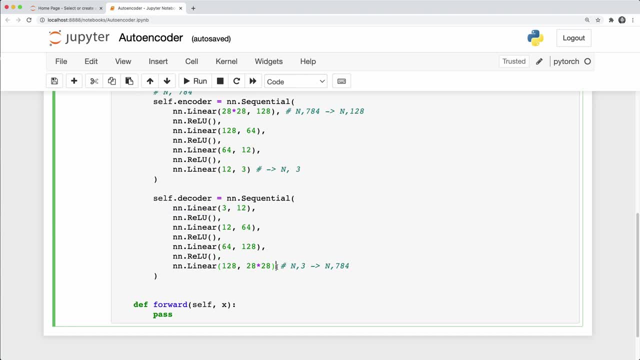 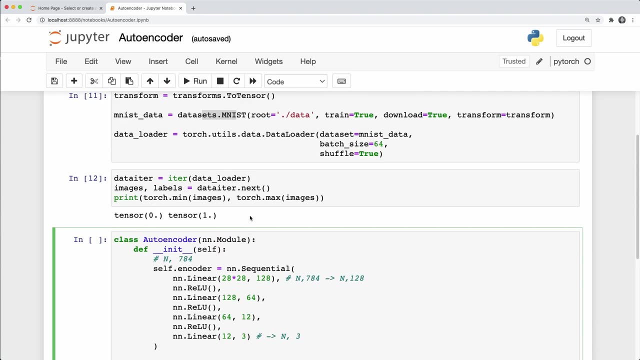 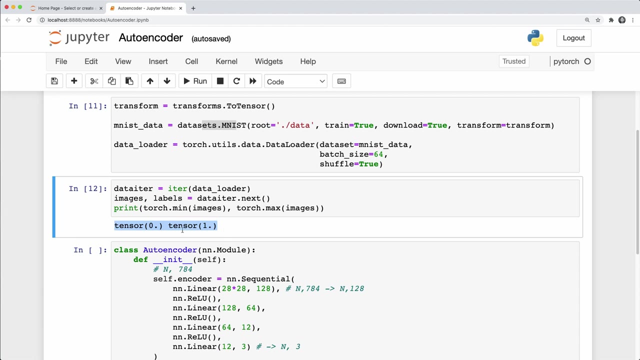 functions in between. And now for the last layer. this is actually important. So here we have to apply another activation function. So let's go back to our data set and have a look at this. So we know that our images have values between: 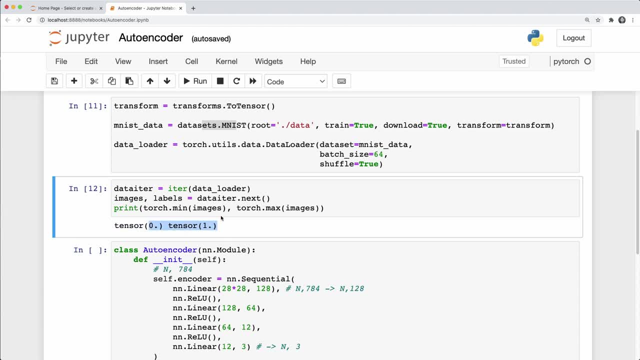 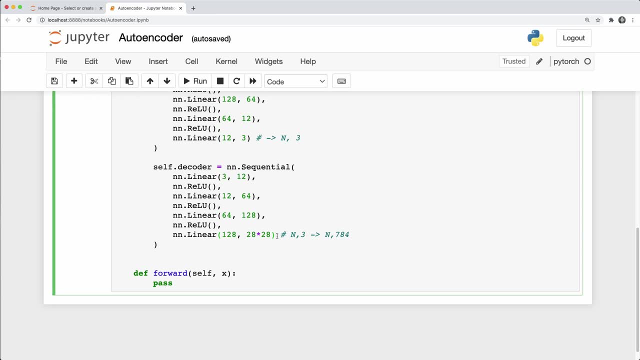 zero and and one. So we now we need an activation function that puts the values in exactly this range. So in this case, the $1 million question is: which actuation function do we need to get outputs between zero and one? So this is the sigmoid function, so we get this by. 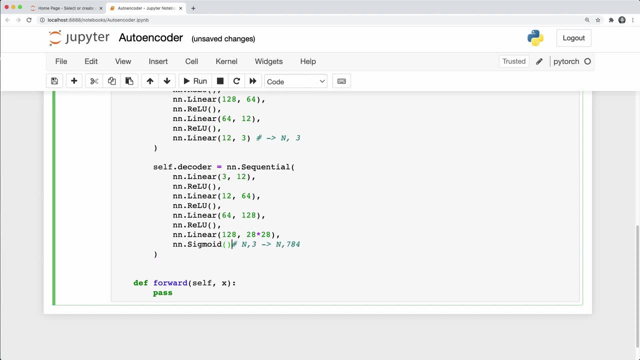 saying nn dot sigmoid. So this is what we need as last layer. So keep this in mind. So now we have our encoder and our, our encoder and our decoder, And in the forward pass we simply apply both of them. So we say: encoded equals self dot. 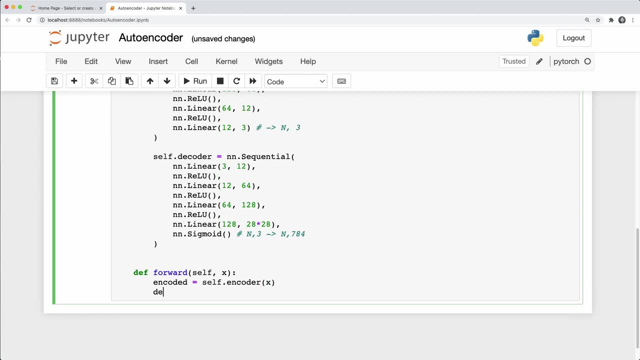 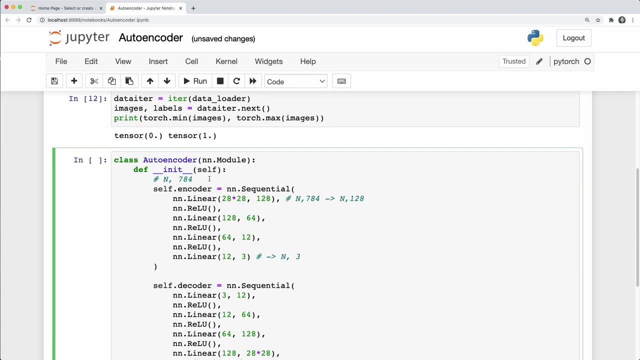 in coder and this gets x, And then we get the decoded again by calling self dot decoder and this gets the encoded as input And then we simply return the decoded image again. And, yeah, this is all we need for our encoder class. So as a note here: 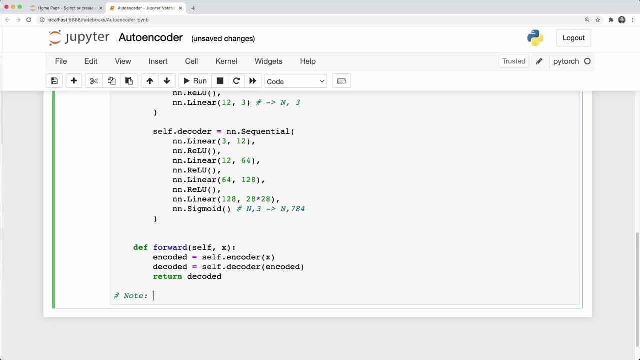 note. keep the last layer in mind. For example, let's say our, our input images are in the range minus one and plus one, then we don't need the sigmoid here. So in this case we, for example, want to apply the ton age function And this: 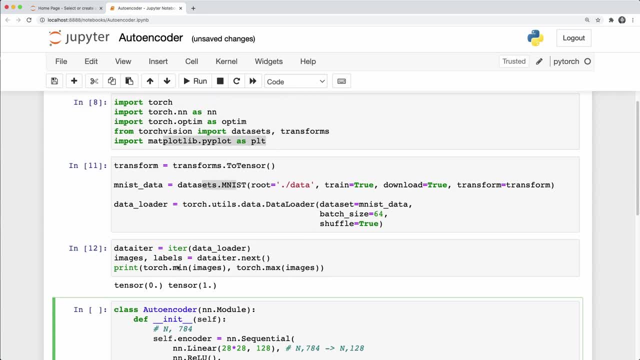 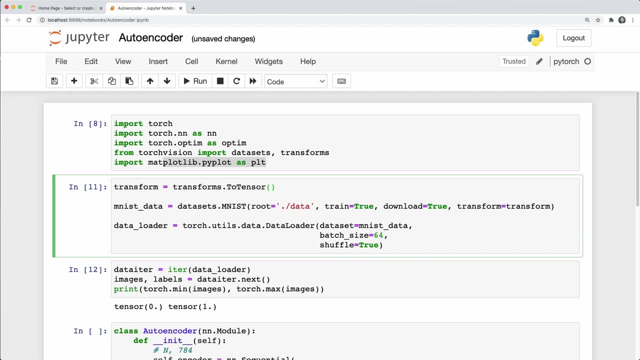 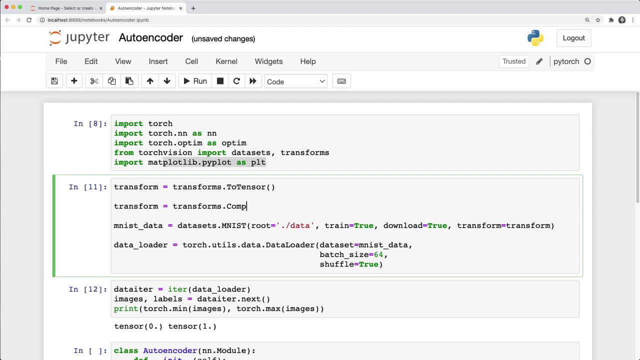 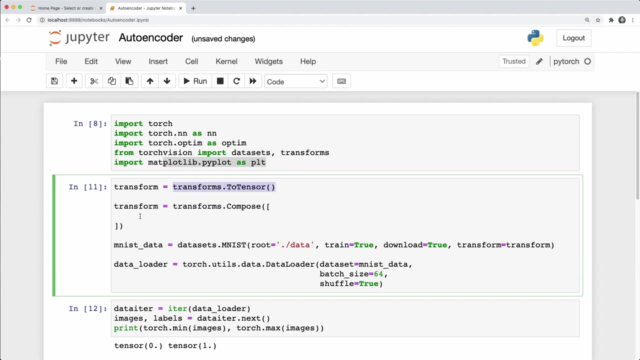 might actually very easily happen if you apply a normalization here. So let me quickly show you how to do this And that's why I pulled this out. So let's say our transform is transforms dots, and then compose, And here we can give it a list. So the first one is again the tensor transform. 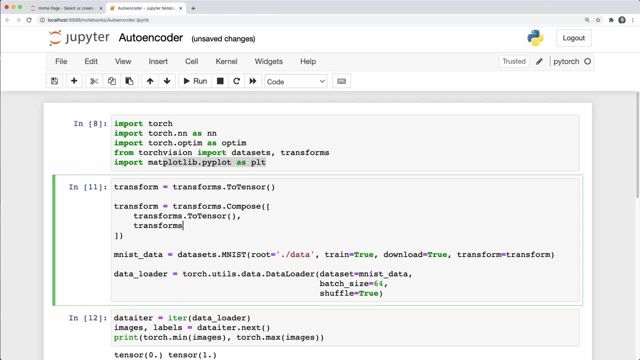 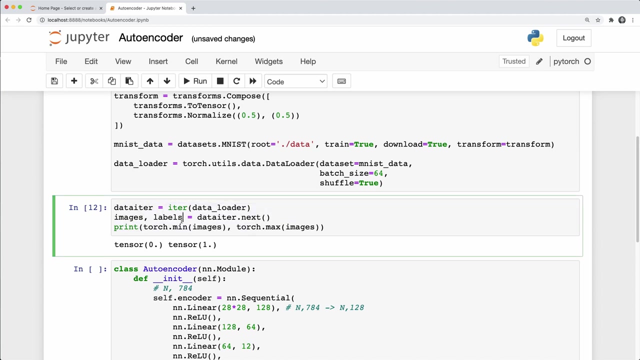 And then we also apply transforms, dot, normalize, And here we want to use point five for the first dimension, And for the other dimension we want to use point five as well. So now, if we comment this out, so let's actually run this and then also run this again and have a look at torch min and max. 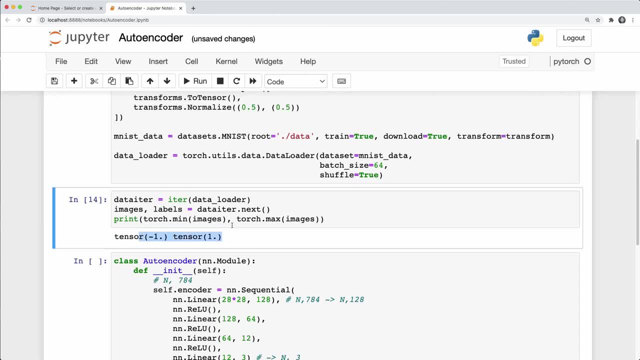 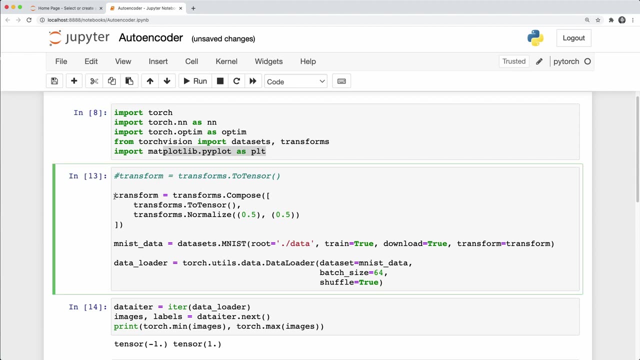 then we see we get the range from minus one to plus one. So that's why we always want to analyze our data first and want to know what are the ranges, And then here we might use, for example, the ton age. So keep this in mind. So now I will comment this out again. And we simply 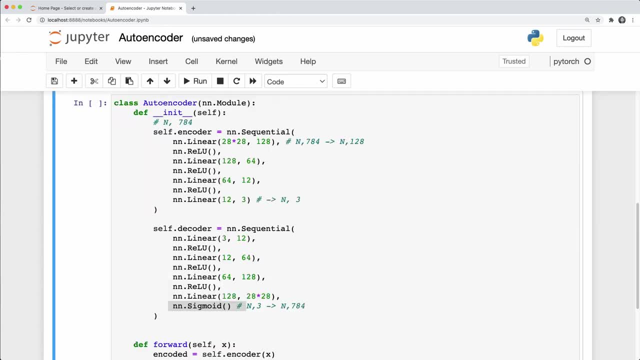 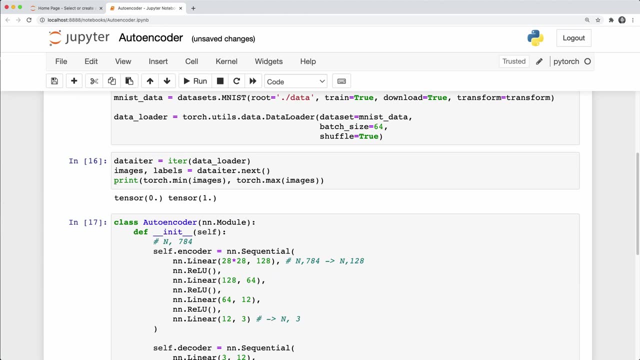 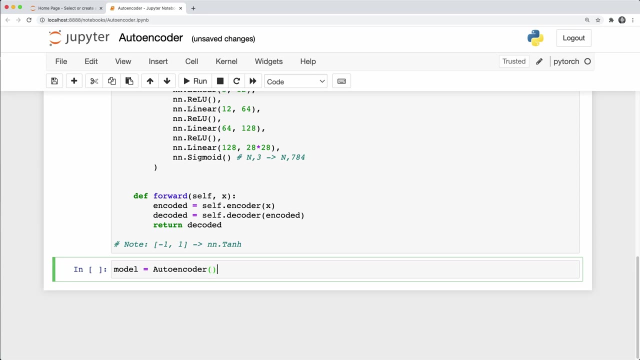 use the trends to tensor transform, And now we have our images in the range zero and one again. So now here, we created our encoder. So now we actually want to set this up, So we create a model and say: this is our encoder. then we also need a cry, cry Tyrion, And I already told you that this. 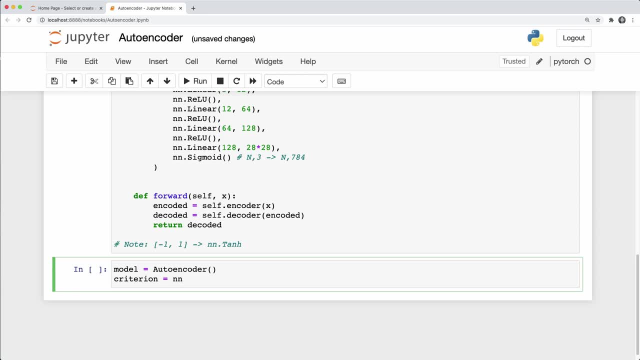 is simply the mean squared error loss. So we get this by saying n? n dot m s e loss. And we also need a optimizer. So optimizer equals torch dot optimum, And here let's use the Adam optimizer. And we want to optimize the. 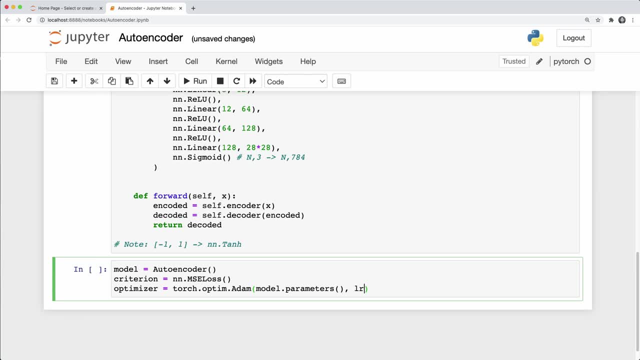 parameters of our model, And we also need a learning rate. So here let's use one e minus three, so point 001.. And also, if you want to, you can give this a weight decay, So weight underscore DK equals. and let's use one e minus five, So you can play around with these numbers. 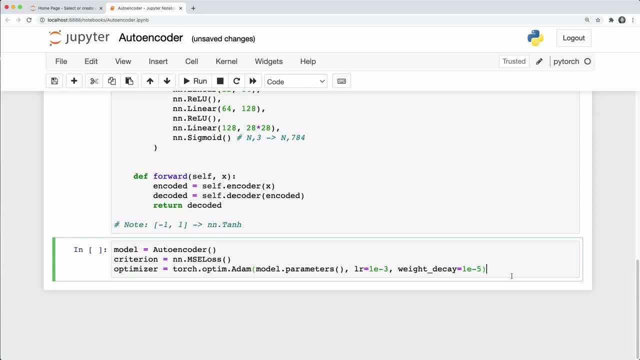 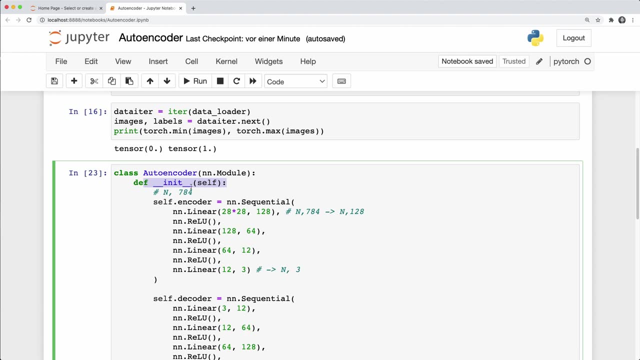 and see which performs better. So let's run this cell And now we get an error. And this is because in our init function of course we have to call super dots, underscore in it and initialize the superclass. So I always forget this when 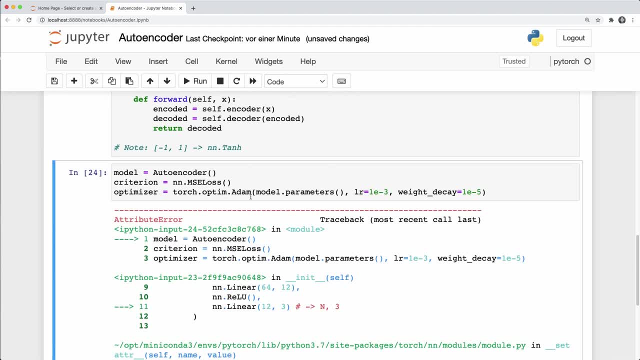 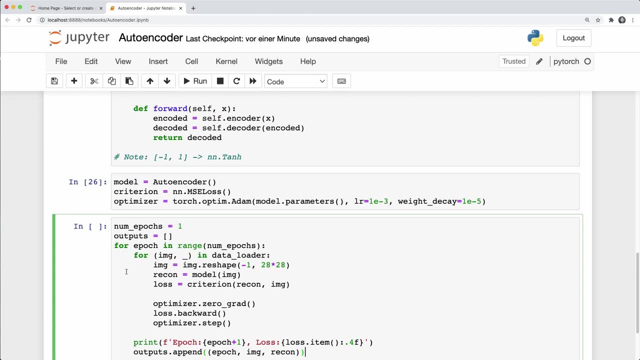 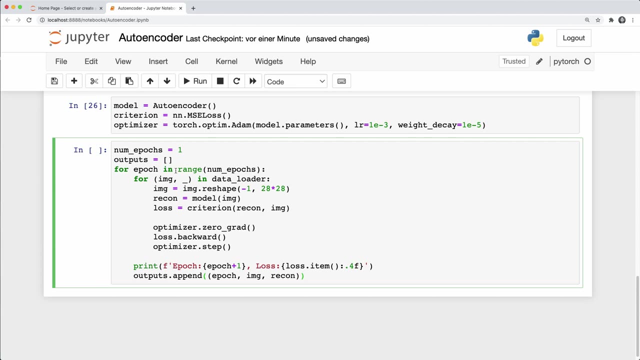 I record tutorials. So let's run this again And let's run this again. And now this works And now we do the training. So for this I simply copy paste this here. So if you don't know how the training loop works, then I will link another tutorial here where I explain this. So basically, 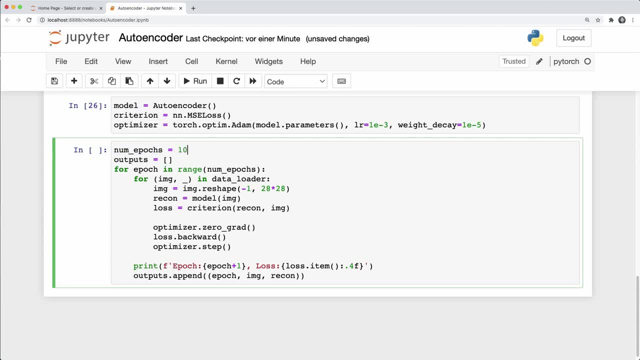 we define the number of epochs And then here I will set this to 10. Because this might take a few minutes to train if you don't have a GPU. So you can of course increase the size if you want to have more accurate values, then we create a list to store the outputs. then we iterate over the epochs. 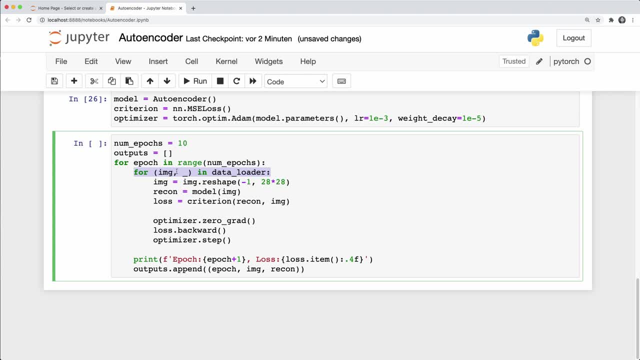 And then we also iterate over our data loader. And now here we want to reshape the images in our first example, because the images are in the shape 28 comma 28.. And we want to have this in size 784.. So that's why we apply this. then we call the model and get the reconstructed image. 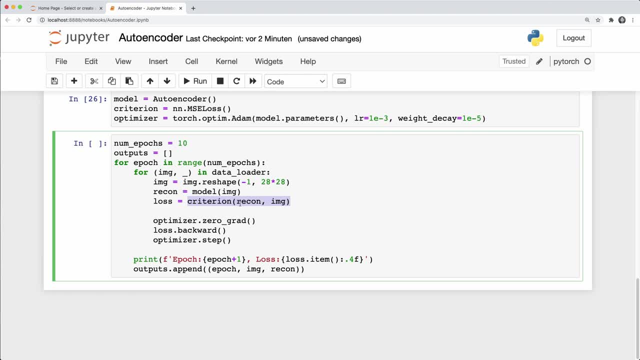 then we call the criterion With the reconstructed image and the original image and calculate the mean squared error, And then we have to be careful to always zero our gradients and then call loss backward and an optimizer step, And then we also want to print the epoch and the loss after each epoch. 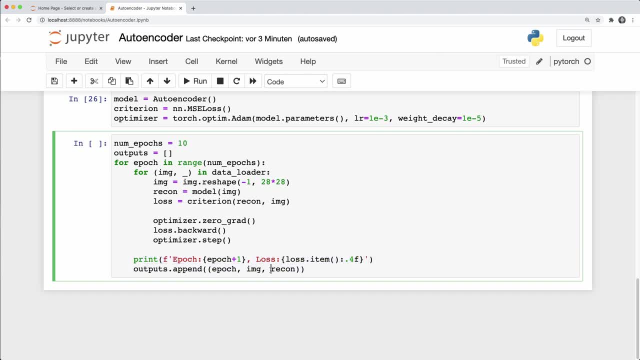 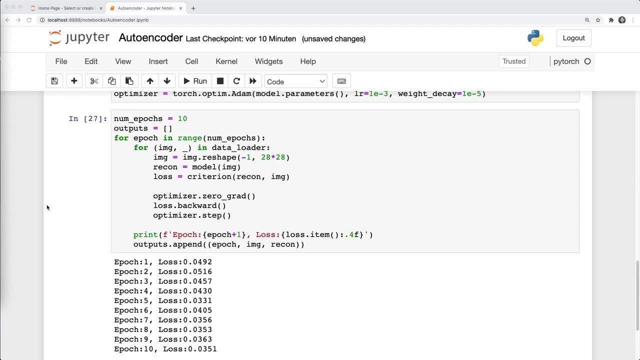 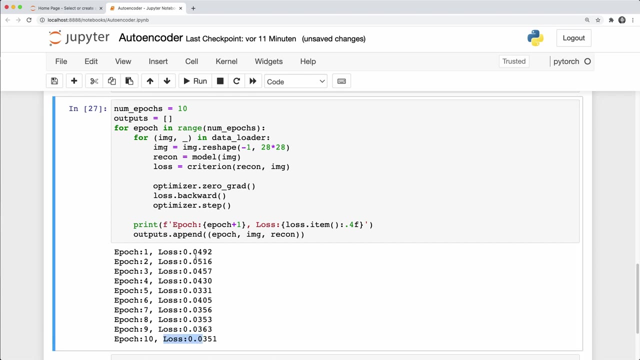 And we want to store the epoch, the image and the reconstructed image in the outputs list. So let's run this All right. so training is done and our loss slowly decreased. So it's still not that low, but maybe you might want to increase the number of epochs, But it's working And let's actually 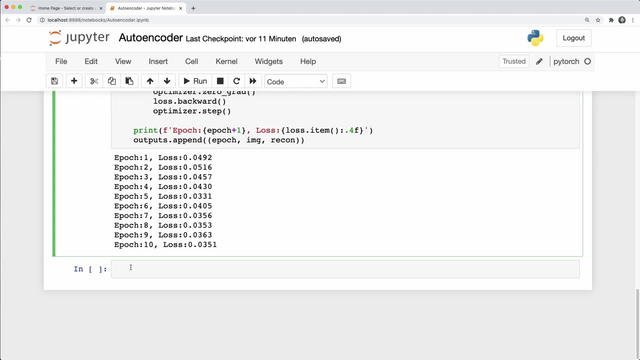 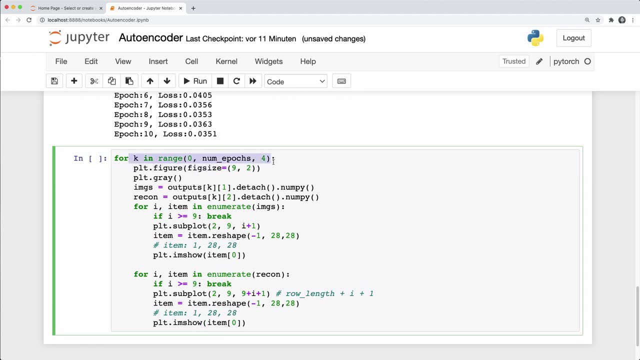 have a look at how the reconstructed images look like. So let me copy and paste a simple function here that will plot the images. So we will plot the images every fourth epoch and create a figure, And then we get the images and the reconstructed images from the outputs array. that 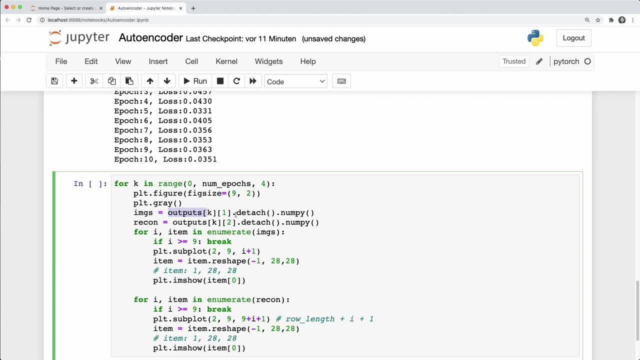 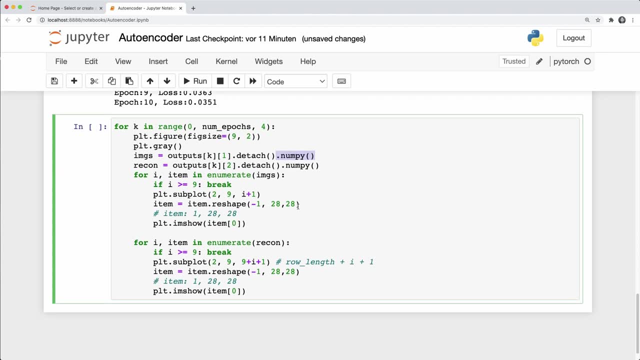 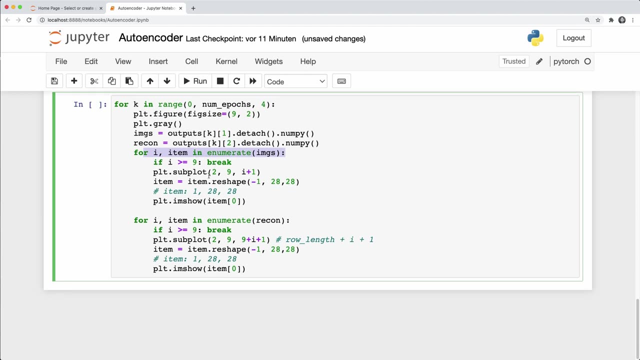 we start, And this is a torch tensor, So we want to call detach and then convert it to a numpy array here for plotting. And then we iterate over the images and plot the first nine images, And here we want to be careful. So here again we want to apply the 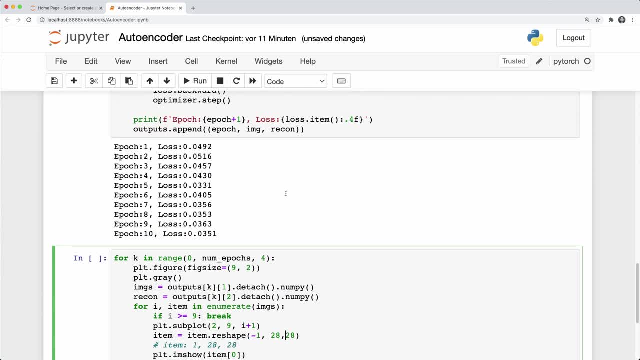 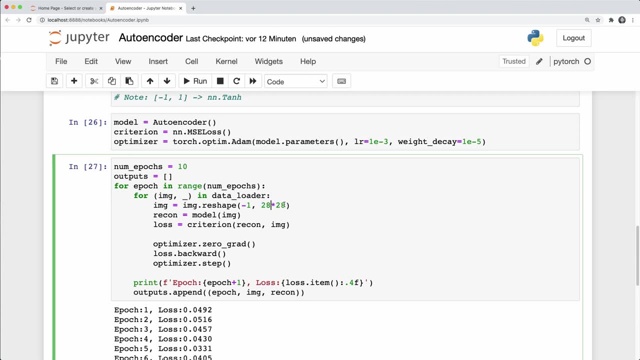 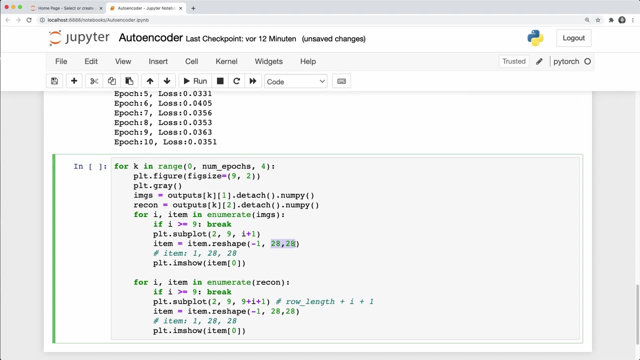 reshaping again in the reverse direction. So here we went from 700, from 28 comma 28, to 28 times 28.. And here we want to go in the do the opposite, So we do 28 comma 28.. And then we simply 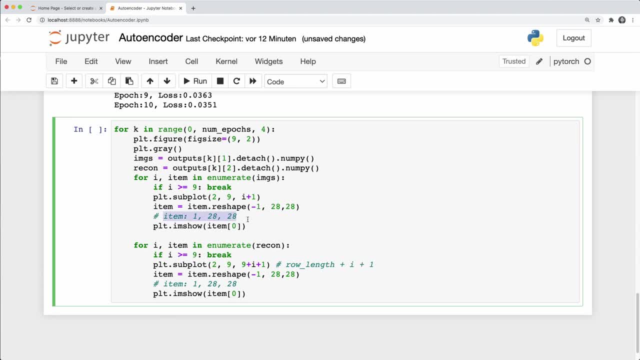 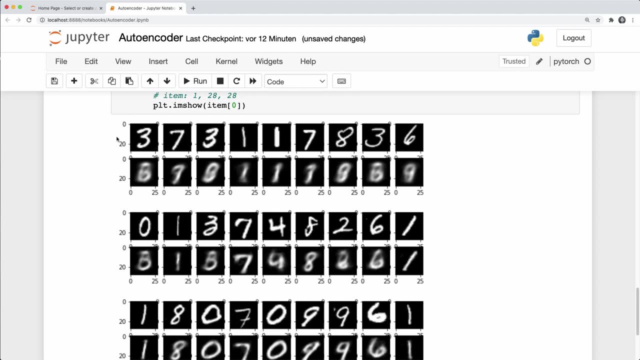 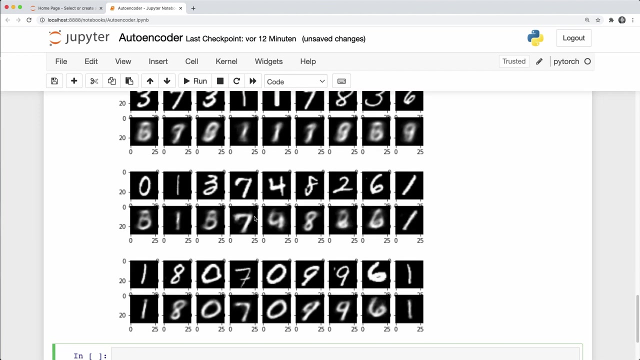 plot this. So here our data has to be in this format. So let's run this And we see. so this is after the first epoch and we can almost assume the correct number, but it's very blurred And then it's getting better after the next four epochs. 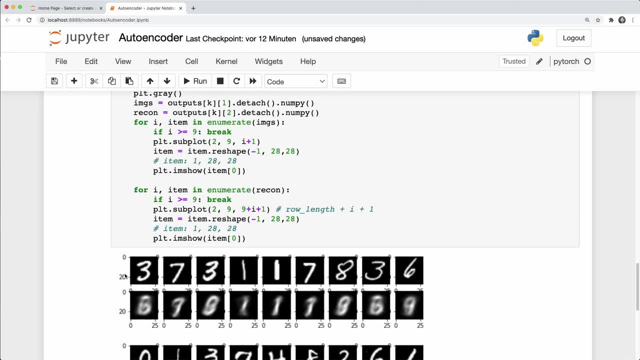 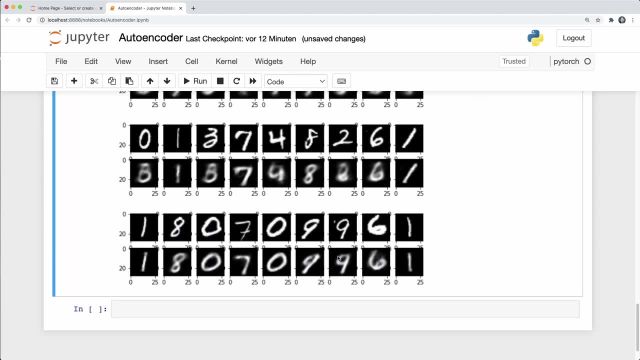 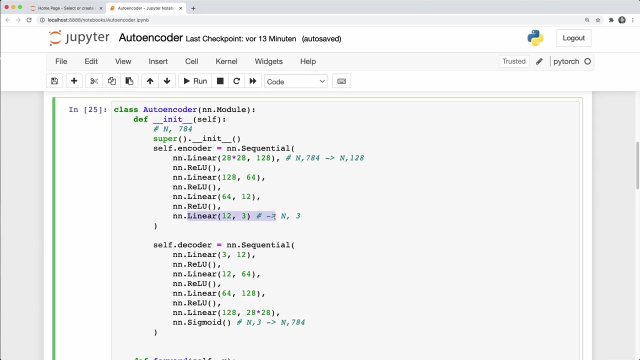 And I think this is after eight epochs. So then we see this image and we see that the result is still a little bit blurred, but it's actually pretty good, So we can detect which number this is, And I think this is pretty good for a simple linear layer that reduces. 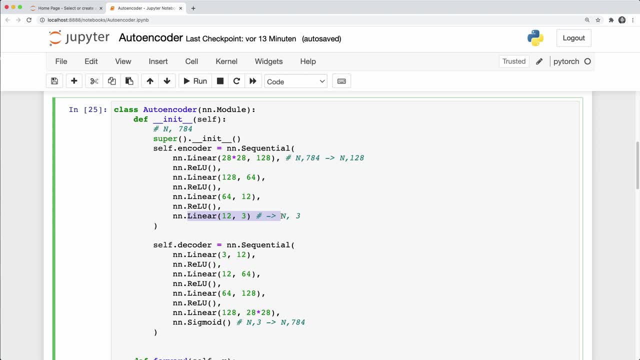 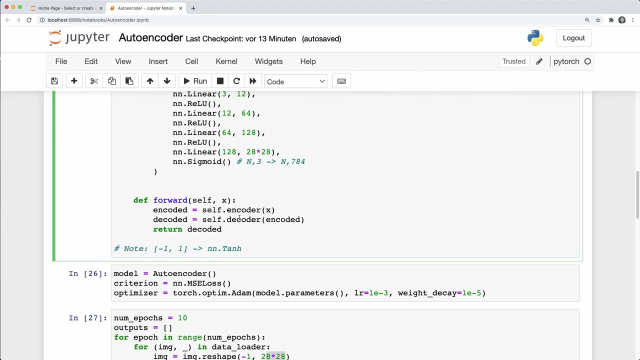 to the size, to only three output layers, So I think this is pretty cool. Yeah, so this is the first example I want to show you, And now we want to use a convolutional neural network and see if we can improve the performance. 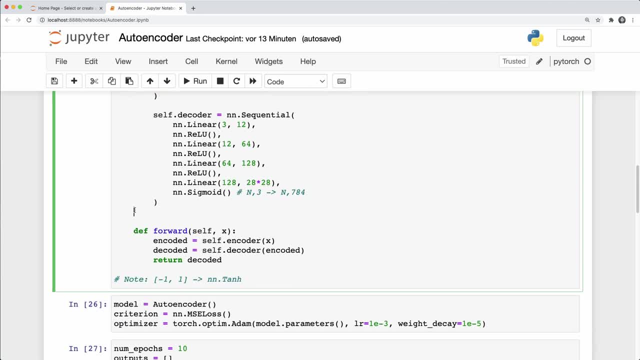 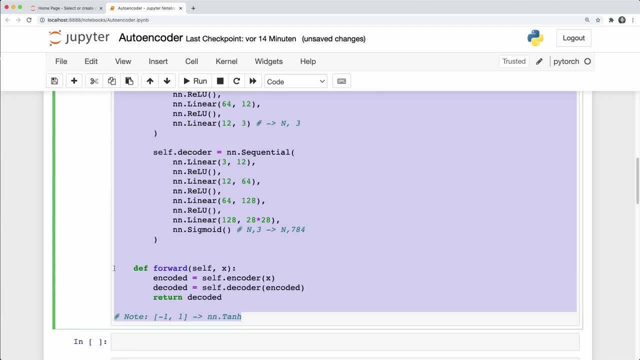 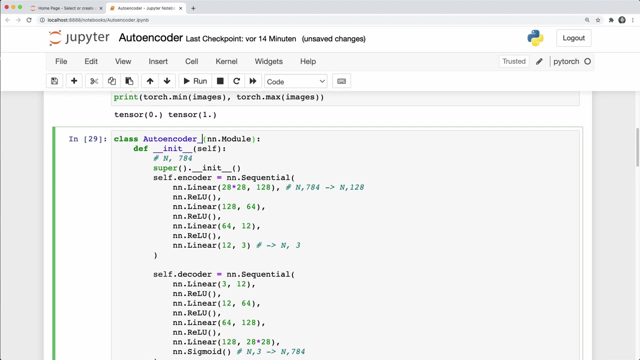 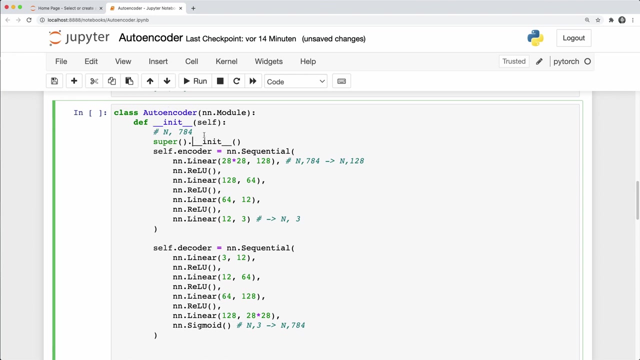 with this. So let's run this again and create a new cell, And then let's actually copy and paste this class and put it down here. And for the first auto encoder, let's rename this to auto encoder, underscore linear, And this will be our CNN auto encoder. So here we do. 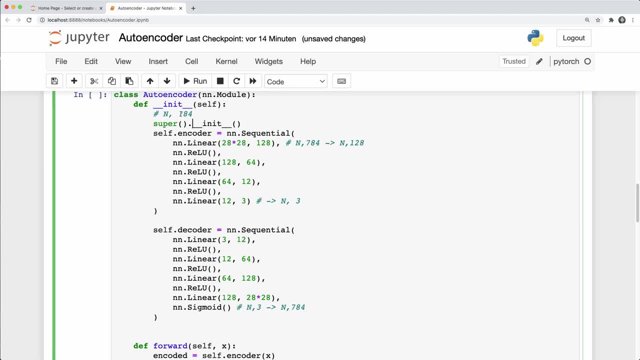 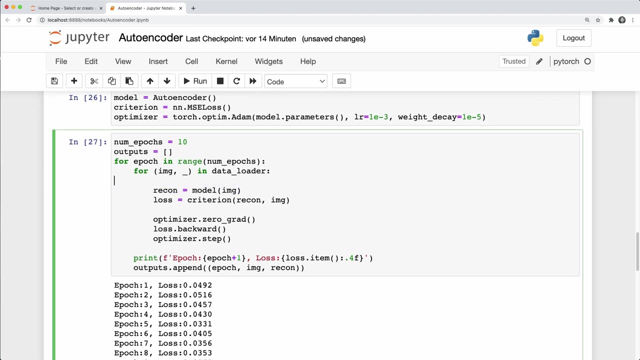 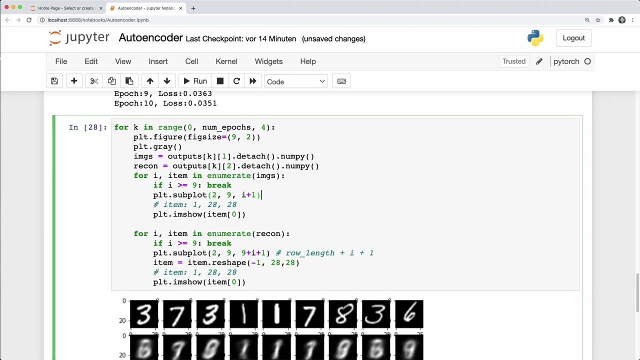 the same thing. And now the first we want to do- it's now here- we actually put them in as 28 by 28.. So in our training function, training loop, we can remove this reshaping, And also later for plotting, we can remove this as well. So let's do this first, And 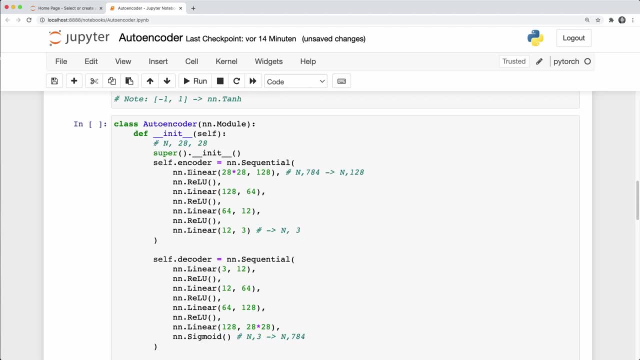 yeah. So now that's able to another Sister. and now we want to see that we've already loaded the. now we can continue here. So now, instead of linear layers, what we want to have here is convolutional 2d layers. So here we can say nn, dot, conf, and then to D, And here we have. 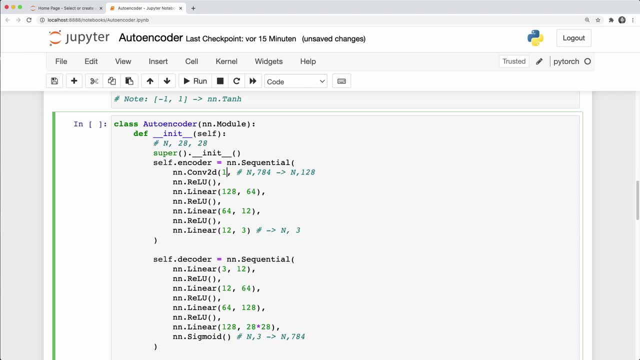 to give it input channel and output channel. So this is one, and then you can play around with this size. So let's use 16 as the first number of output channels, And then we also have to give it a kernel size. So here we use three, then we can give it a stride. So 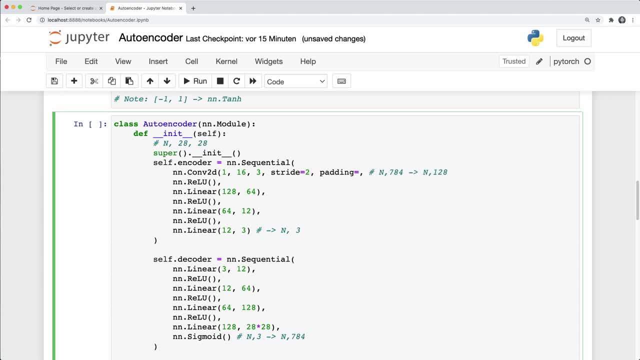 this is two, and let's use a padding equals one. So this is our first convolutional layer, And then as well, here we want to apply really activation functions. then let's create another convolution, then again the relu, And then let's use another convolution, And then we 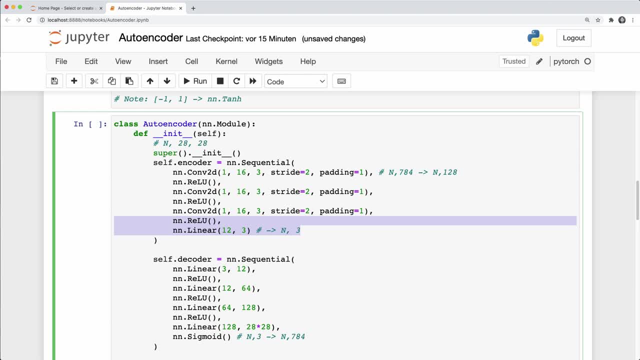 can actually. let's get rid of those here. So we only want to do three passes And now let's simplify this a little bit and get rid of this. So now it gets a little bit tricky, because now you have to be careful to get the correct shapes and the correct input and 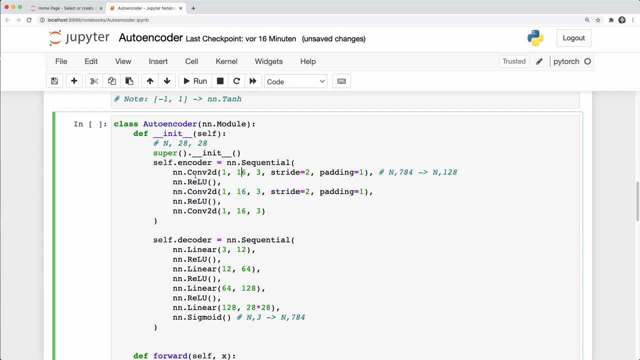 output channels. So again, if you don't know how these convolutions work, then I will link the tutorial about the CNNs where I explain this. So actually, let's inspect the input and output size. So the input for this is n by. 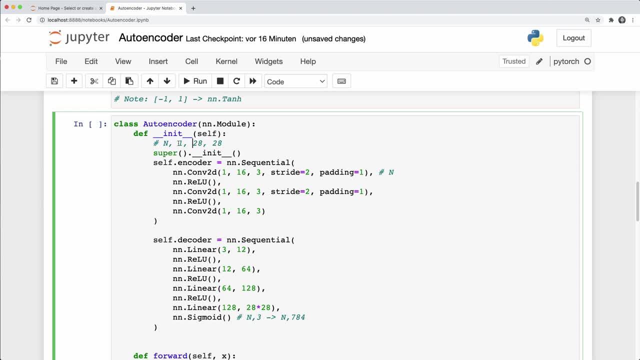 one by 28 by 28.. So this is why our first input size is one, And then after that we get 16. And for the size, we get 14 by 14. So we reduce the size of our images by 50%. 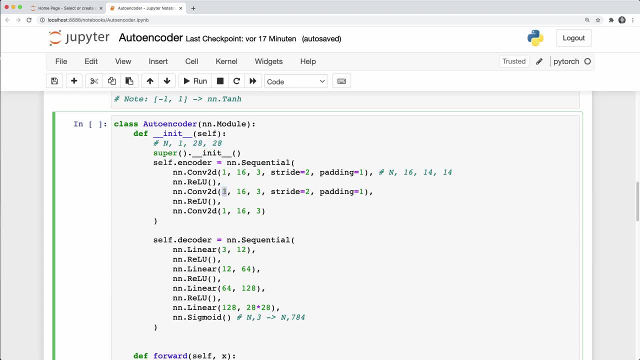 And and then for our next one, as the input size we have to get the output channel size of the previous one, So this is 16. And then here we can actually increase this and use twin 32. And we will keep the rest. And then again let's have a look how this will look. 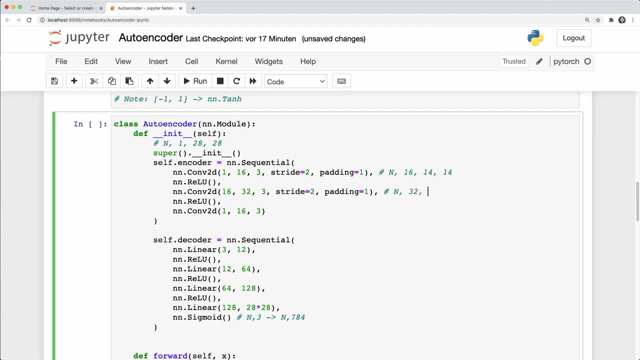 like. So this will be n by 32 by seven by seven. So again we reduce this in half, And then again we use a real, and then again a convolutional, and this will have 16. Let's actually increase this again, So 64. So here we have 64 output channels, And then here: 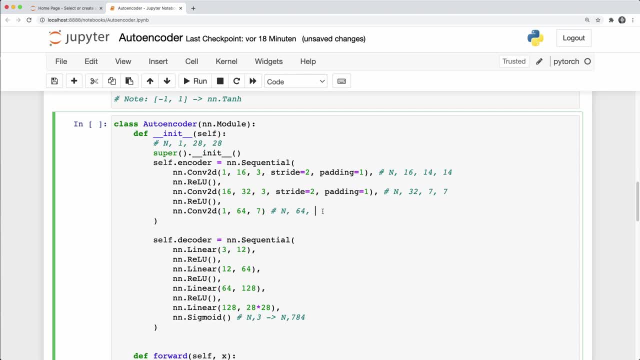 we want to use. let's use seven, So we have one by one as the output size of our image. So basically, only one pixel, But 64 channels. So we increase the channels but we reduce the size of the image. So now, 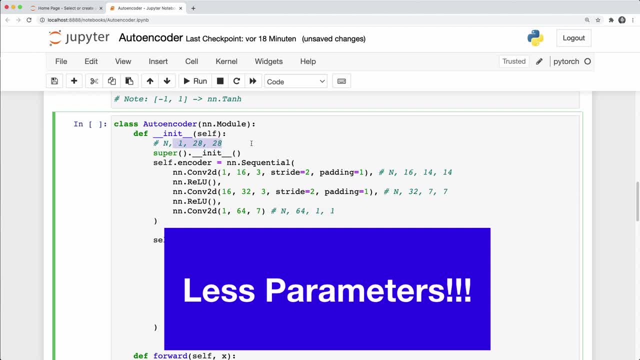 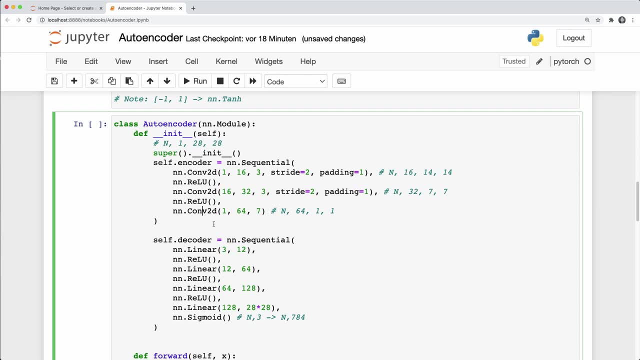 this has far more parameters than this size. So this is our encoded version, And now we want to go in the backwards direction with the conf, transpose two D layers that I mentioned. So here let's copy and paste this to know with what size we are working. 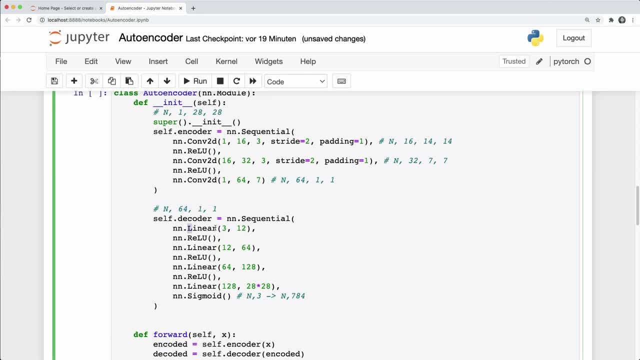 here. So now we apply the nn dot con, transpose to D. And now here we again have to switch the sizes, and here I made a mistake through copy and paste. So here this input size must be the output size of this one, So here we have to say 32.. 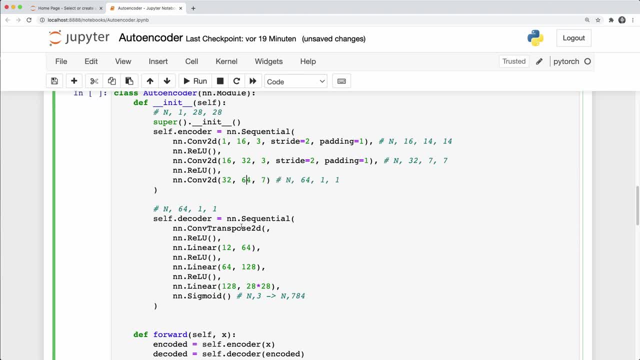 two, and then 64 and seven, And here we do the opposite. So we have 64 input channels and 32 outputs channels And the kernel size is seven. So this will give us the size n by 32, by seven, by seven, So like we have here. so this is correct. Then again we use a real. and now let's use 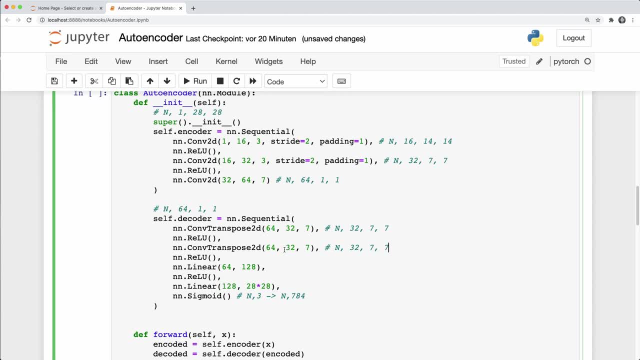 another conf to D conf, transpose 2d, And here we switch this convolutional layer. So here we have 32 as the input and 16 as the output and a kernel size of three. And now if you run this, then this will actually give you a size of n by 16, by 13 by 13.. 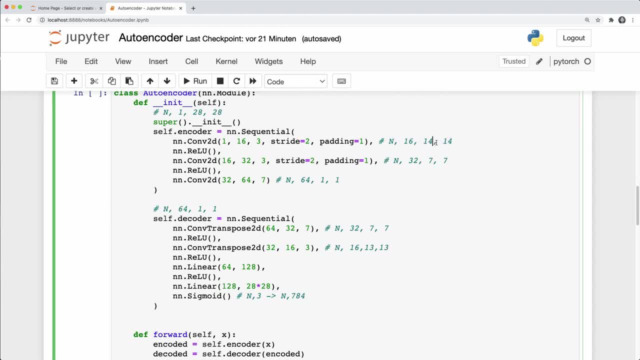 And what we want. we have 16 by 14 by 14.. So we need plus one. So this is a little bit tricky, So I recommend to play around with these ones and have a look at what they generate. And now, in order to compensate this, we can give it a parameter. And here let's, actually let's. 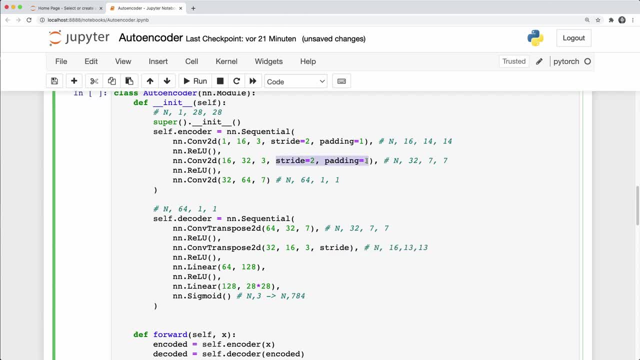 say, let's use the exact same stride and padding that we have here: stride equals two and padding equals one. And here we have the same stride and padding that we have here: stride equals two and padding equals one. And here let's actually let's say let's use the exact same stride and 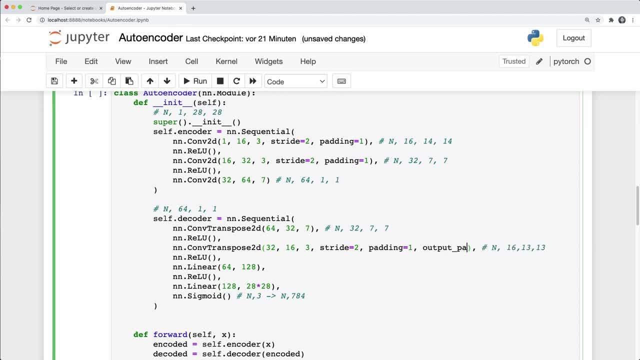 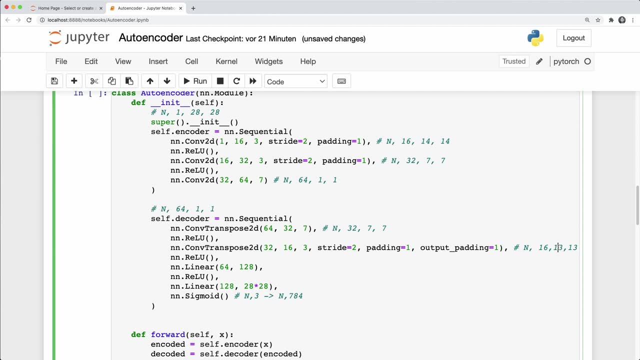 padding equals one, And then we can say: output padding equals one, So this will put zeros in it, so that you get 14 by 14. now- So yeah, this is a very important thing to know- to use the output padding parameter. And now again, we use the relu function and then we use another conf: transpose 2d. 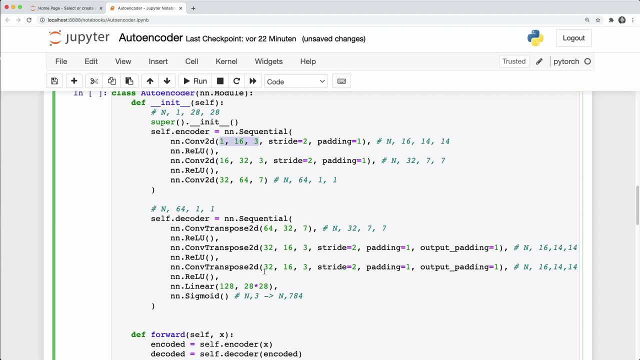 and here we have to revert this one, So as the input we use 16.. And as the output we use one. And then again we have the same kernel size, the same stride and the same padding, And now here will happen the same thing. So if we don't use this, then we get n by one, by 27, by 27.. 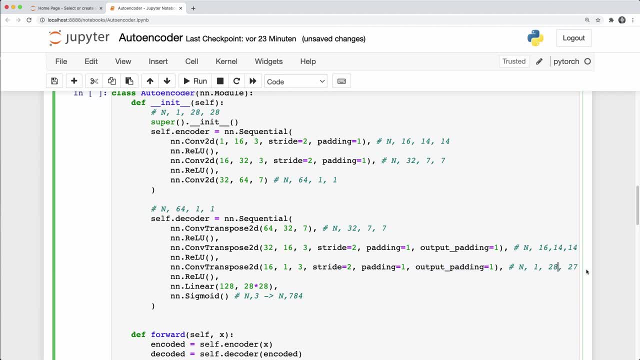 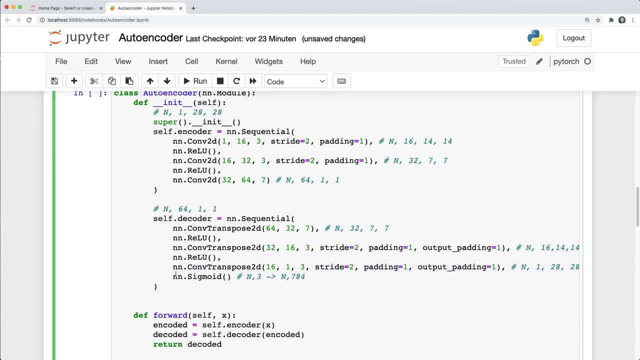 So then again we need the output padding, and then we get n by one, by 28, by 27.. And then we don't need these anymore. And again, as the last layer, we want to have the sigmoid. So the same as before, And now this is no longer correct. So yeah, this is how we implement a. 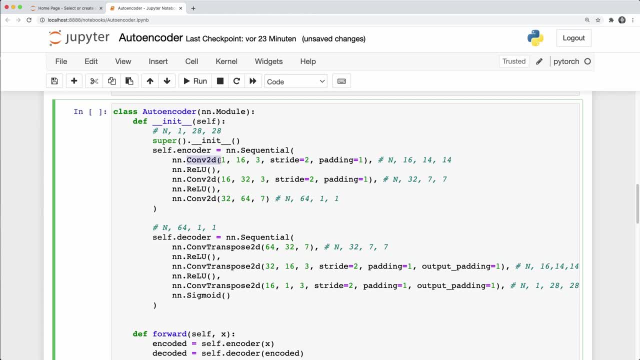 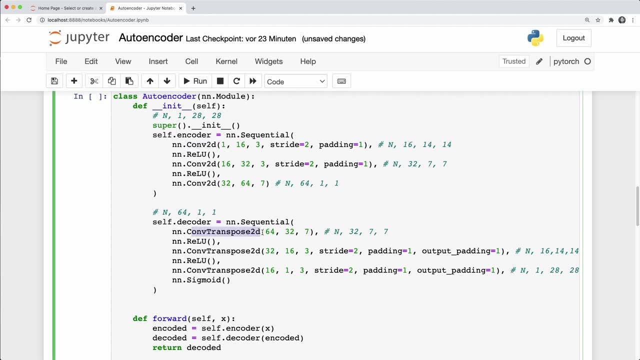 auto encoder with convolutions. So we need the convolutions And then in our decoder we use conf, transpose 2d And be aware that you use the correct shapes and also maybe use a output padding if necessary. So let's run this. And here I actually want to mention one more. 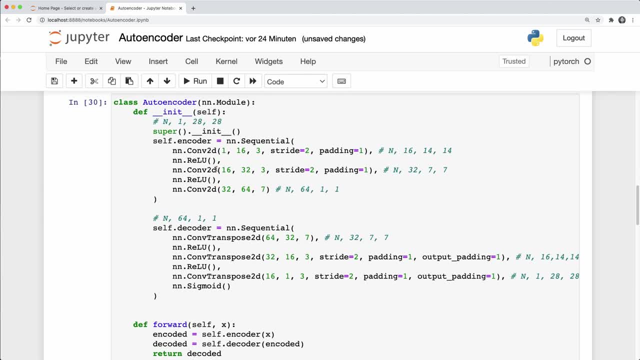 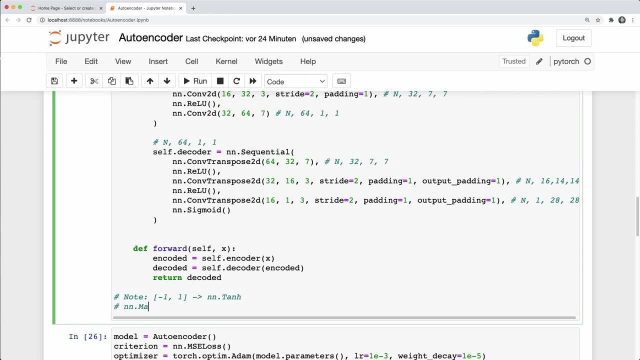 thing. So a lot of times in convolutional neural networks you use the max pool 2d function, So nn dot, max pool 2d. this will essentially reduce the size And to revert this there is also a function that is called nn dot max pool 2d, And this will essentially reduce the size. and to revert this 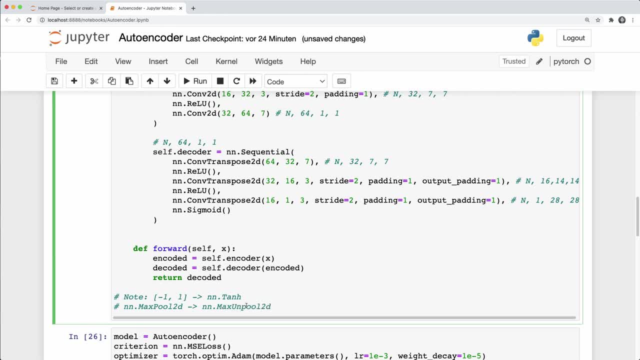 there is also a function that is called nn dot max pool 2d, And to revert this, there is also a max on pool 2d. So this is what you might want to use in the decoder then, But you don't need to. 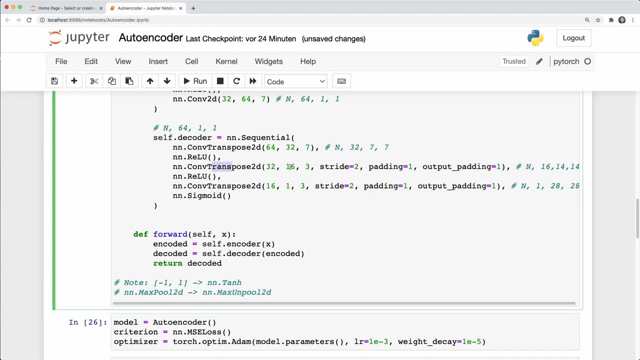 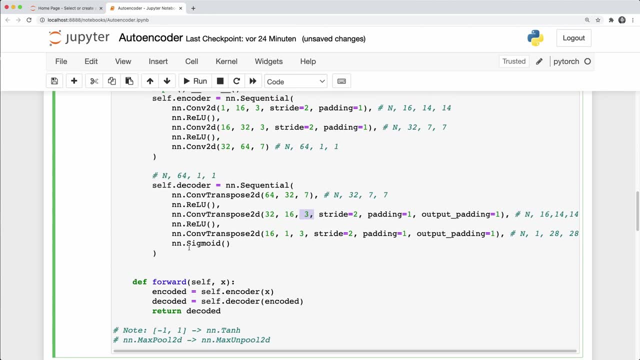 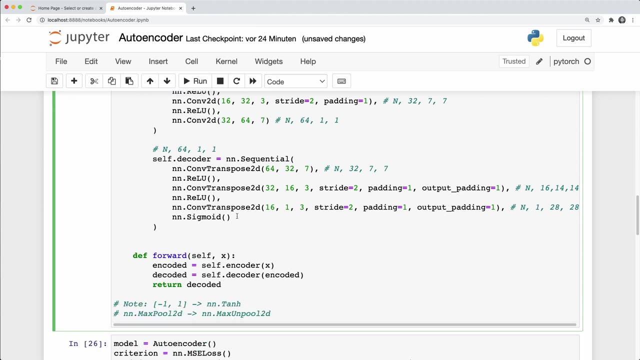 do this. You can also, for example, play around with different stripes and paddings and kernel sizes. The only thing you want to make sure is that at the very end, you get the same output shape as you had in the beginning. So yeah, keep that in mind. And now let's run this. And now. 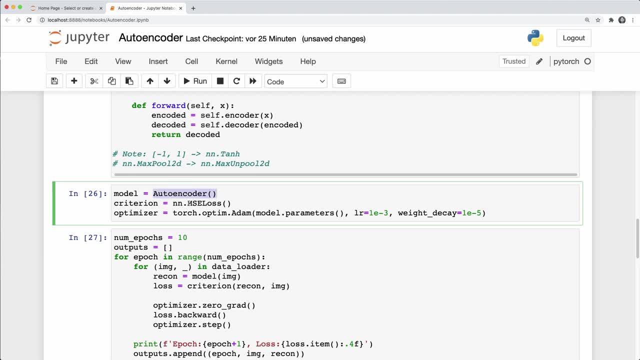 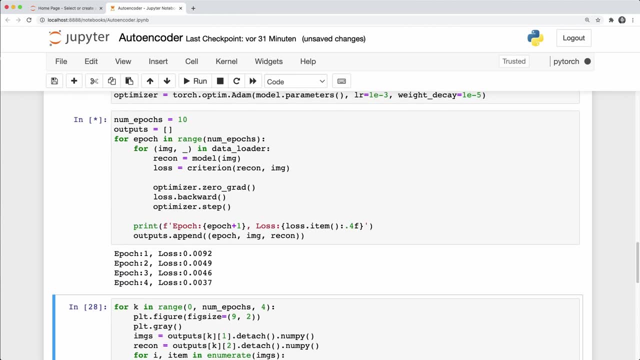 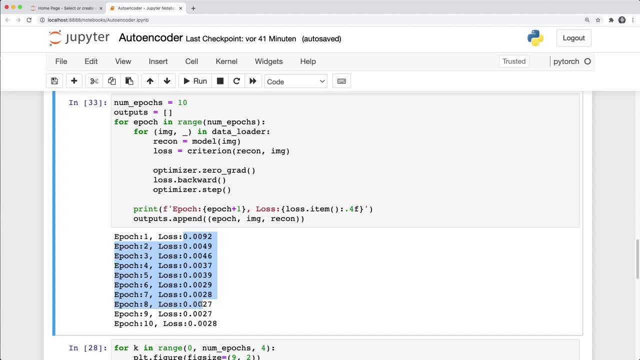 again our loss decreased And now this time it's much better than before. So I guess before we had point 03 something And here we have point 00 something, So this is much better. So, yeah, we can see that our CNNs. 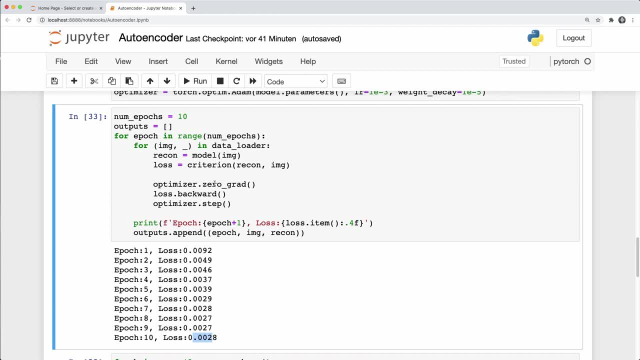 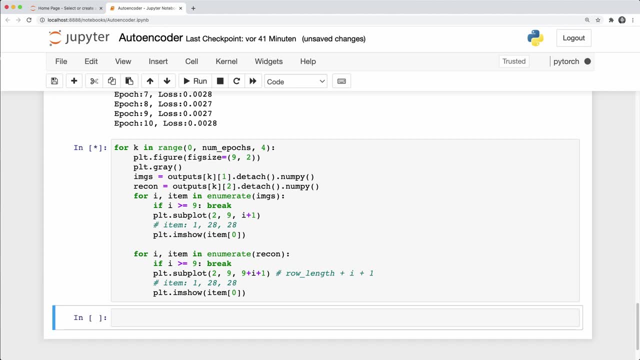 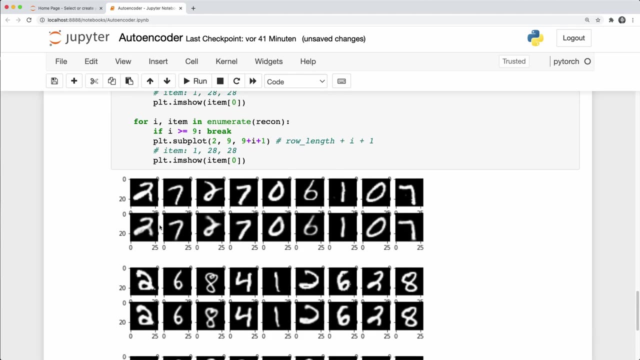 usually perform much better than a simple feedforward neural net with linear layers. So let's actually run our plotting loop again And let's plot some example reconstructions. So we can see that after the first Epoch it's a little bit blurred, but it's already very good. 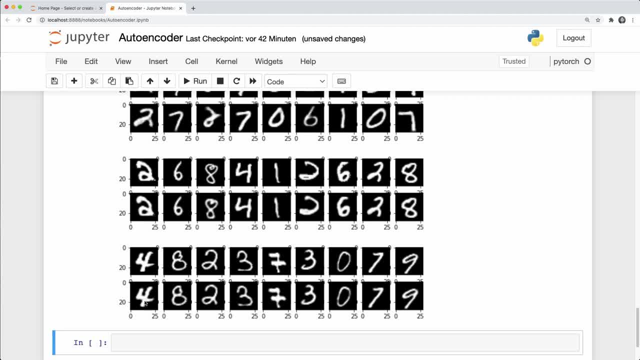 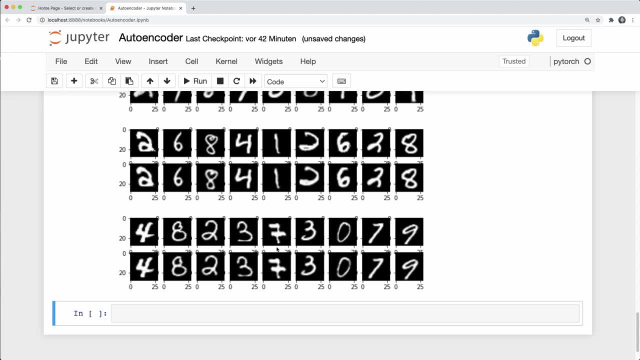 And then this is after the fourth and after the eighth epoch, And we can see that already here the reconstructions are a lot more uniform. the first epoch is a lot more structured, And then the second epoch is pretty good. So, yeah, I think it's almost the same image. So, yeah, this is really cool.